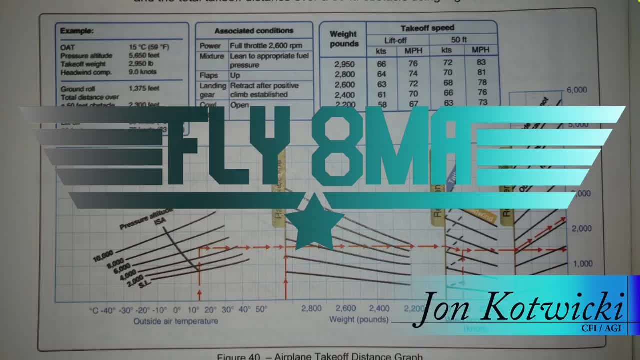 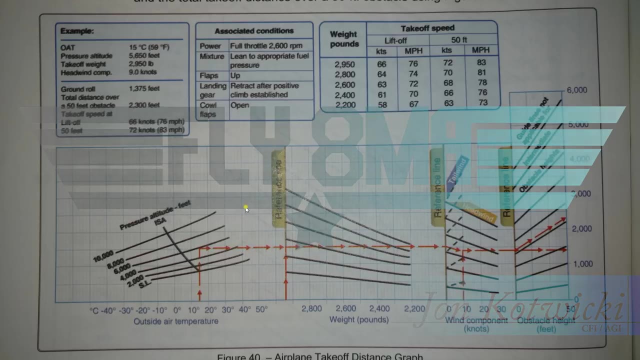 Hey guys, what's up? John from flymycalphacom and today we're going to be looking at airplane takeoff distance graphs. So I know these are kind of complicated looking. It's pretty archaic, but it's something you do need to know flying some of these older airplanes and especially for your written exam, You need to know how to do these. So we're going to go ahead and explain this to you. I know it was pretty complicated to me at first when I started looking at these, when I first started flying. However, I am going to, over the next 120 seconds, explain to you exactly how to use these charts and less than two minutes from now, it's going to make perfect sense. 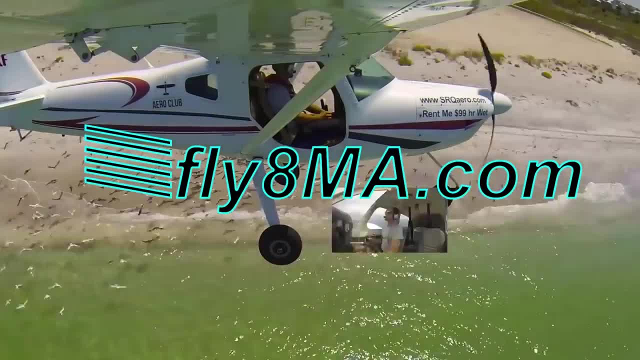 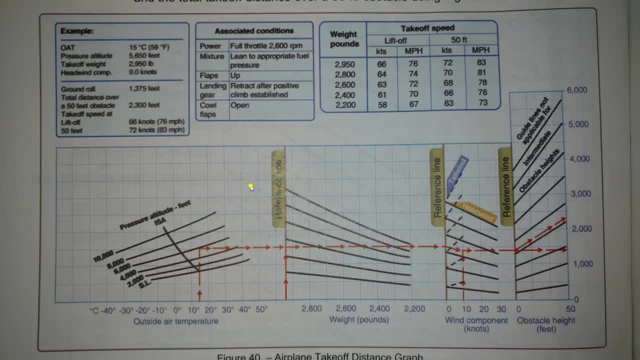 All right. so there's always going to be some givens here, So we're always going to have to know our pressure altitude, our outside air temperature, the weight of the aircraft, the wind component and the obstacle height. Those will all be given to you on the test or you'll figure them out in real life. So the next thing about these charts is we have these things called little reference lines and they kind of trend in. 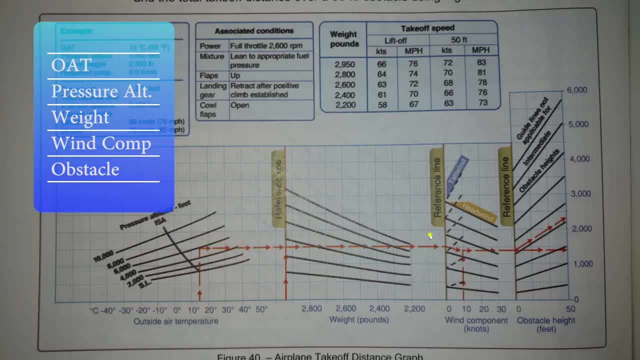 these different curves and the purpose of these is for us to follow them when we're making our calculations. I'm going to explain that here in a sec. So if you happen to actually intersect one of these lines, you could follow it on up or follow it on down, But if you're in between them, you'll just follow the general trend. So if we come over here and intersect right here and we're going to 2600 pounds, we would follow the trend lines down to our 2600 pounds, meet the roughly where that trend would be and then proceed straight across. So let's go ahead and work through an example here. Our example today is: 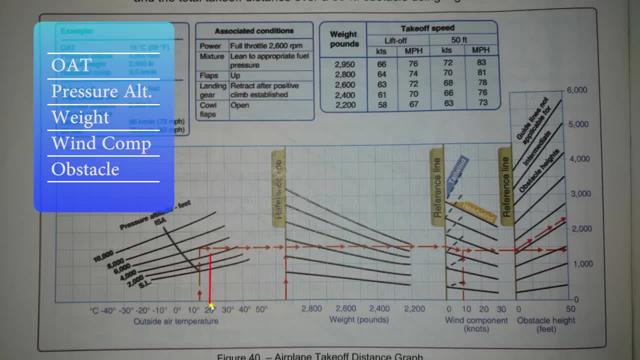 going to be that it's 20 degrees outside air temperature and we have a 4000 foot pressure altitude. So we set the altimeter to 299 or 2 and we got 4000 feet on it. So 20 degrees. we're going to come up to 4000 pressure altitude and we hit that line and then move straight across. We intersect this next line here and we're going to follow the trend lines down to our weight. Our weight today is 2400 pounds, So we're following those trend lines down to 2400 pounds. Again, 20 degrees to 4000. 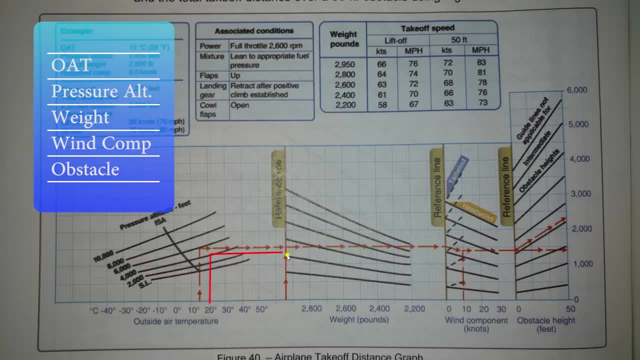 straight across. We hit just above this black reference line. We come down to 2400.. We'll be just above it And then we move straight across from there. Next thing we're going to take into account is our wind component. Our wind component today is a 10 knot headwind, And we can see.